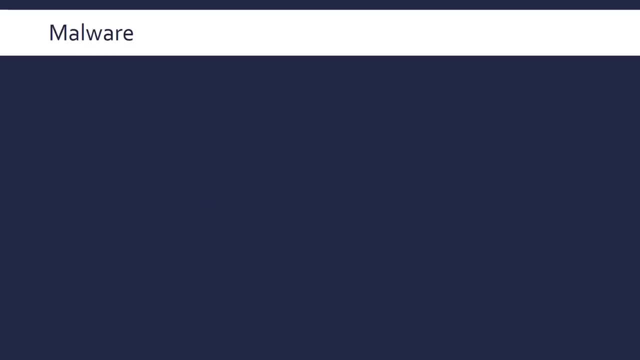 than you'd imagine. I mentioned it just now. we've got a look at malware in a bit more detail, which is an umbrella term for any hostile or intrusive software- some malicious software, in other words- and, as I say, it's used in active attacks. so we're going to look at a few examples of the main examples of malware, most of 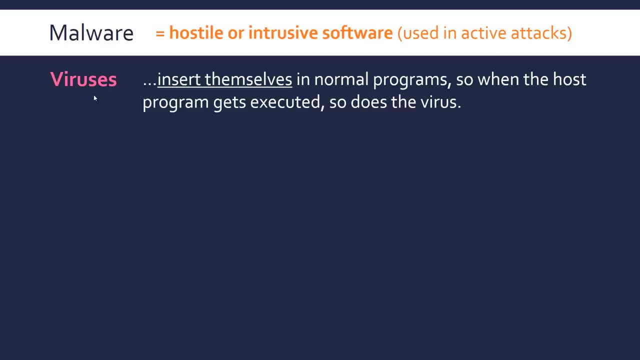 most of these you would have heard of, maybe don't necessarily know how they work exactly. so viruses, first of all. they're unique because they insert themselves in normal programs. so like a virus, when you get ill, inserts itself into your, your body cells, a virus will insert itself into the code of a normal 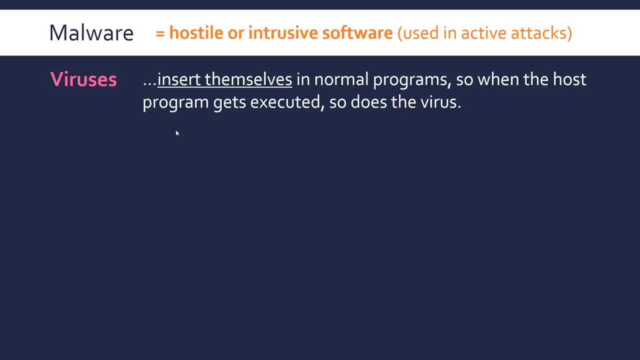 program. so when this host program- a program that's been infected- gets executed, when you run it, the virus code gets run as well, so it links itself to a program on your computer. something very similar are worms, which like viruses but spread autonomously. so a virus doesn't necessarily spread on its 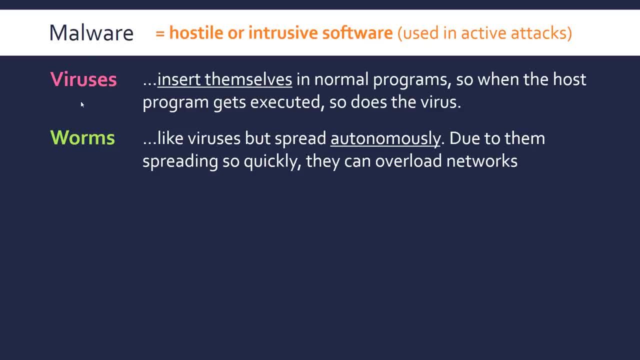 own, but a worm. that's kind of its whole purpose they are is a very fine line between the two, to be honest, and a key characteristic of worms: they often overload networks. by spreading so fast, they kind of spam the network, essentially overloading it. a third type, which is different and this is based on I. 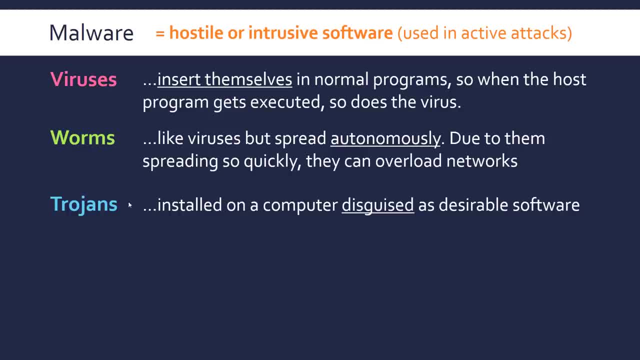 think the Greek story of the Trojan horse. and these are installed on computers disguised as desirable software. so you'll download some software thinking it's something you want like a normal game or a normal program, but actually it's got some malware hidden within it. this Trojan- the next type- is spyware, which collects data. 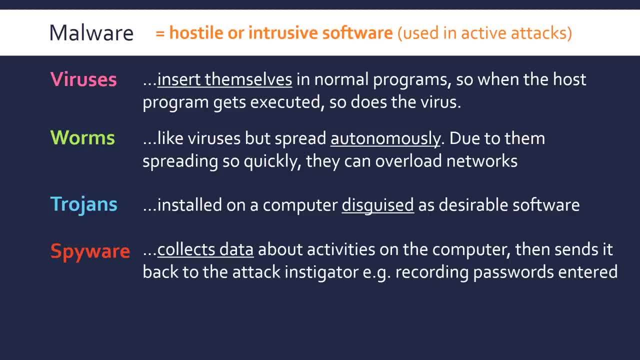 about activities on the computer. so it spies on your activities, as you could guess, when it sends it back to the instigator of the attack. so you know, recording passwords entered. it will track all your keyboards but it will be able to track, you know, your passwords and your details and so on and it sends 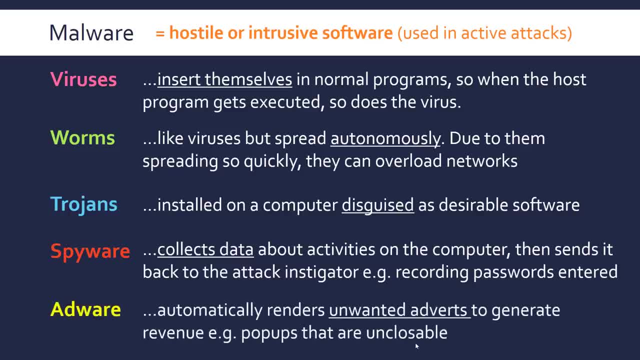 it back to the originator of the attack. the final category look at is adware, which is definitely intrusive software. it's not necessarily hostile, but it may kind of lead you to download viruses and so on. it generates unwanted adverts to make money for whoever started the attack. 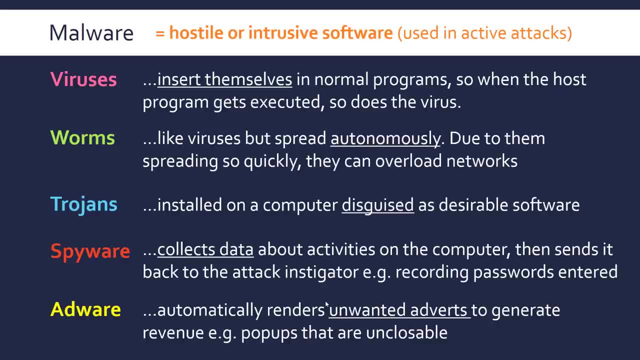 like pop-ups or unclosable. it's probably less common now, but I'm sure you will come across adware to some extent, but anyway, these are the main types of malware you'll come across. we now need to cover some more security threats. it's a lot of learning this video. I'm afraid it is a very interesting topic. 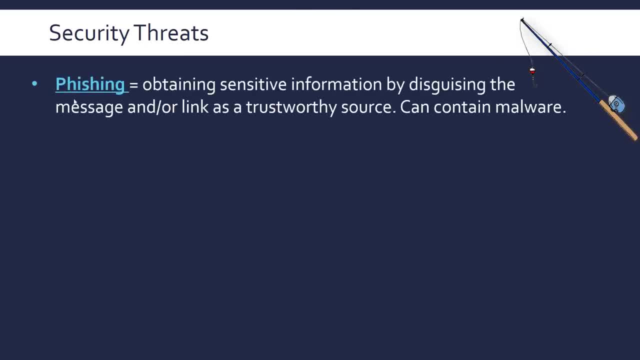 but you need to learn the basics first. so a term that often comes up is phishing, and you may have heard of. this is actually based on phishing. you're kind of reeling someone in by disguising the message in order to obtain sensitive information. so you get an email that looks like it's from your bank or from. 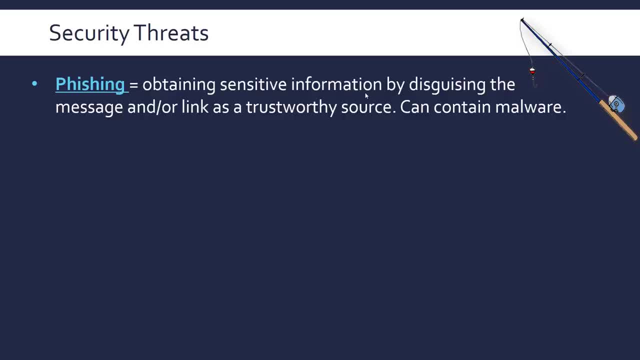 your school and actually it links to something that's pretty different, so it can link to some other malware, and that's what phishing is called. I'm sure you've come across that as well. this is actually, in particular, an example of phishing itself, isn't you know? it's not done by a programmer, it's not code, it's. 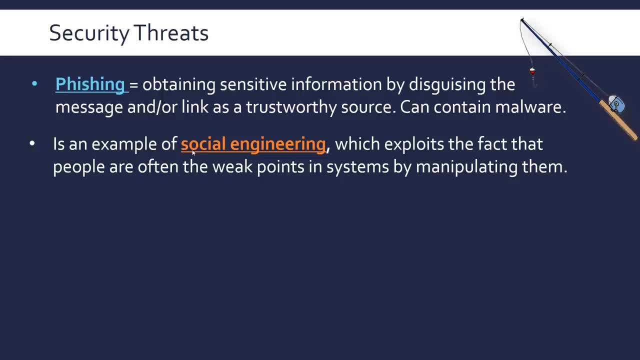 example of actually trying to manipulate someone through something called social engineering, which is exploiting the fact that often people are the weak points in systems, and so you manipulate people to access the data. another term we've come across is a lot less elegant than any of these methods. you've got to give some. 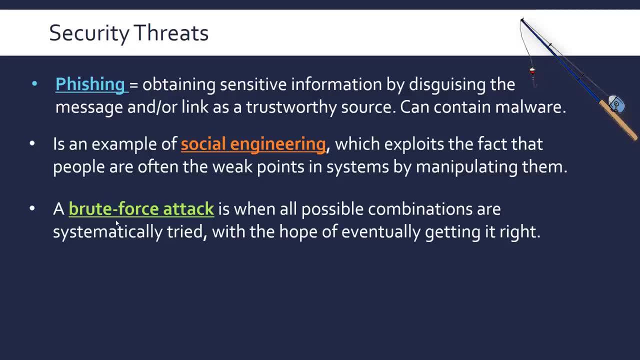 credit to people who do social engineering, however bad it is. a brute force attack is when you literally just try all possible combinations in my hope of eventually getting it right with. in certain cases this is quite a good option in some ways, but you know it gets to a point when you increase the size of passwords or all the information. 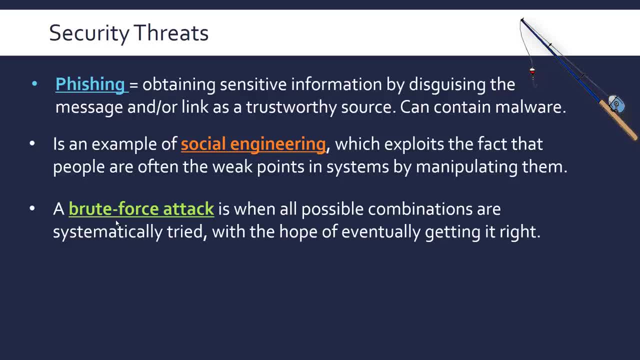 you need to access the system, it just becomes not feasible to do brute force attacks. so, stating the obvious a bit, but the longer the password is, the harder it is, because there's more combinations to try, and so adding more steps to the login can also reduce the chance of a brute force attack working. lots of you. 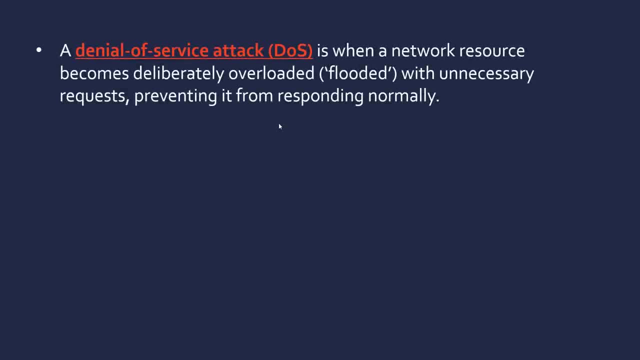 would have heard of denial of service attacks, and this is when an error resource becomes deliberately overloaded. so someone's deliberately trying to overload the resource, or flooding a resource with unnecessary requests, preventing it from responding normally. so it talks about the client-server relationship and in this case, a client. 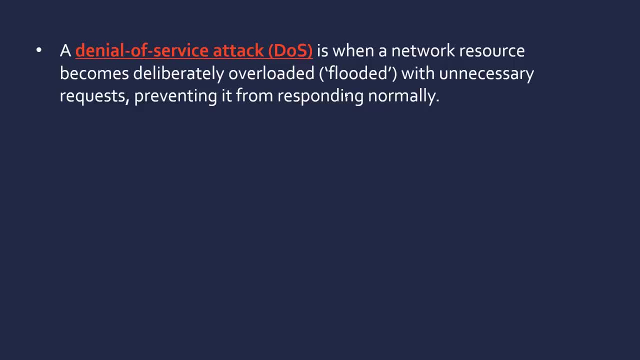 is trying to overload the server by sending so many requests that it can't respond normally to. you know your everyday web accesses and you probably actually heard the term DDoS rather than just DOS, so a distributed attack, which is what the extra D is, for it comes from multiple locations, so multiple sources. 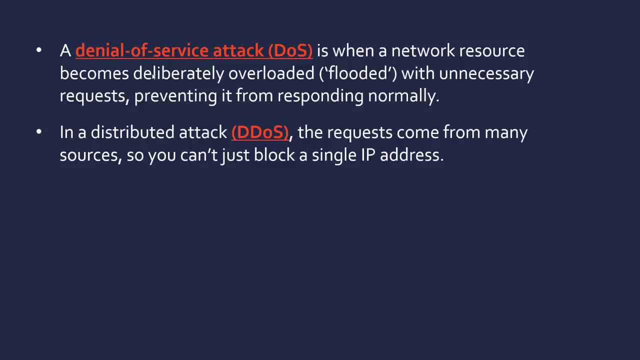 a denial of service attack isn't necessarily from multiple sources, but a DDoS is, and for most web servers it needs to be. it needs to be so many computers that it is massively distributed. so you it does make a hard as well. you can't just block a single IP address because it's coming from so many. 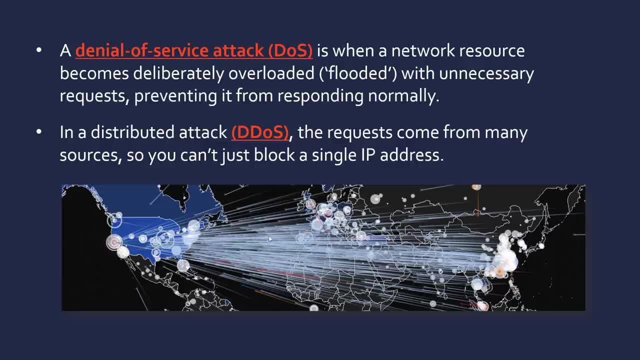 so you can get like live maps of these happening around the world which are quite cool to look at. this is from quite a severe one to, I think, data centers in the US from Asia usually is a few usual suspects with DDoS's and you can see if 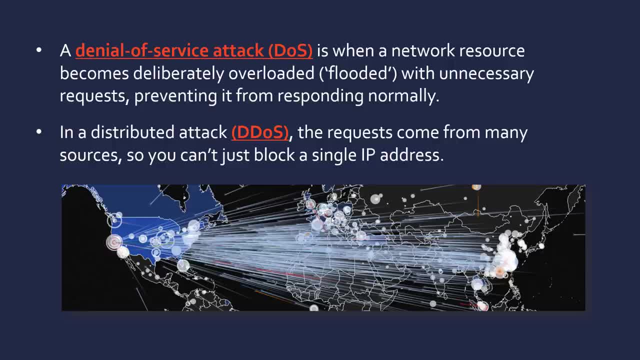 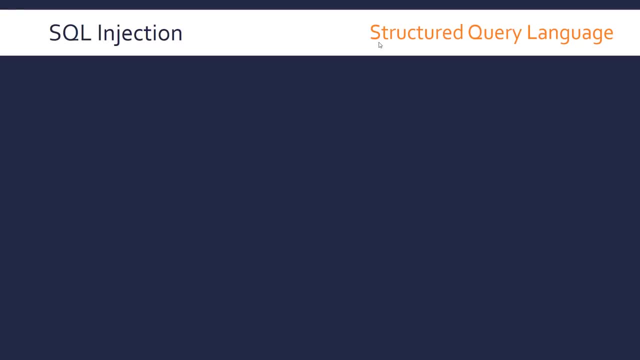 it's coming from those different locations and it's very hard to just block an IP address, and you can imagine that the servers in America would get massively overloaded by all these sudden requests deliberately trying to flood it. So an attack that requires a bit more knowledge is SQL injections, and SQL stands for Structured. 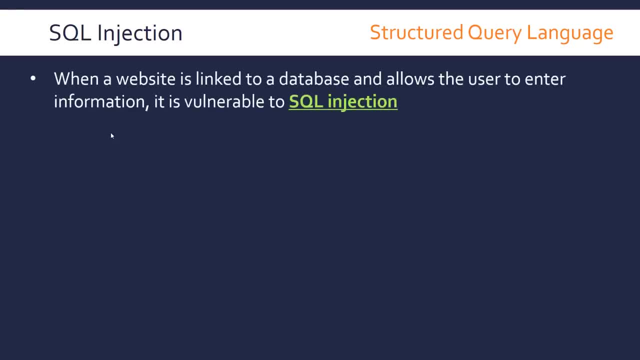 Query Language. It's a language for interacting with databases, and so when you have a website linked to a database, like most websites- in fact, pretty much all websites- and you actually allow the user to enter information, which is not as common but still happens a lot, if you think. 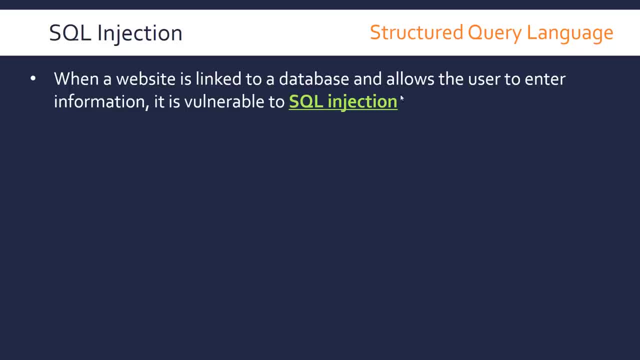 of any websites you search for information or enter details- that's what I mean by this- it's vulnerable to SQL injections. So any website linked to a database with user input and, as I say, SQL is used to interact databases with statements. So, for example, this statement might be embedded in some server side code like PHP. 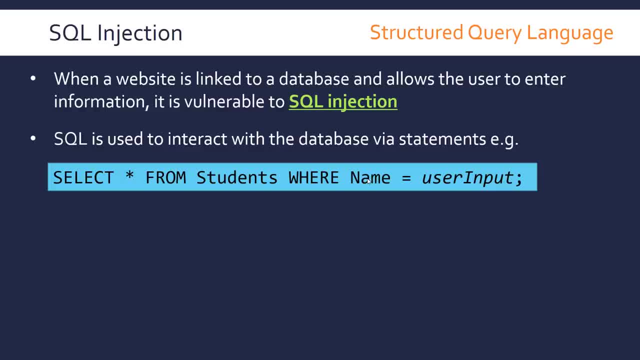 So we're selecting everything from this table where the name which is a column in this table equals something, One variable called user input. so this is what the input of the user would be. So, for example, if Harry was the input in our text box, then this variable would be replaced. 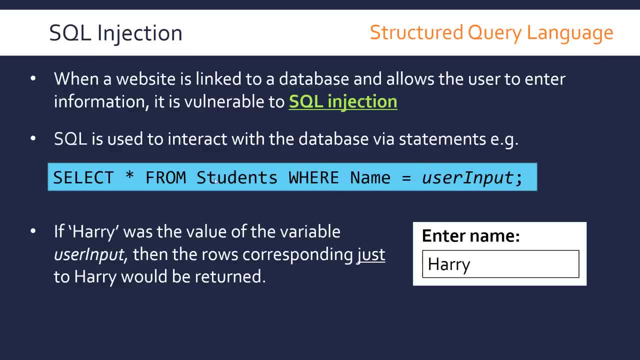 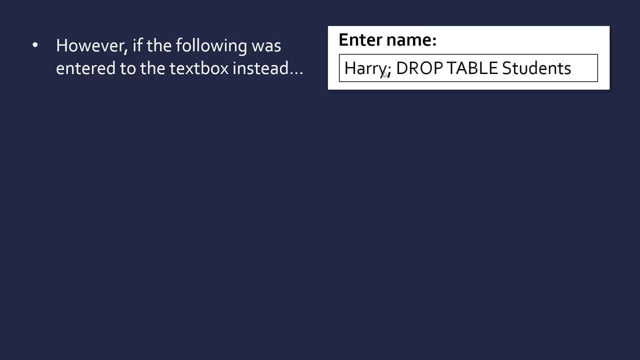 with Harry and just the rows with Harry, would be returned from this statement. So everything works fine in that case. but, however, if we entered the following into the textbook- so not just Harry, we're now putting a semicolon and drop table students, So it will behave like it's been queried twice.